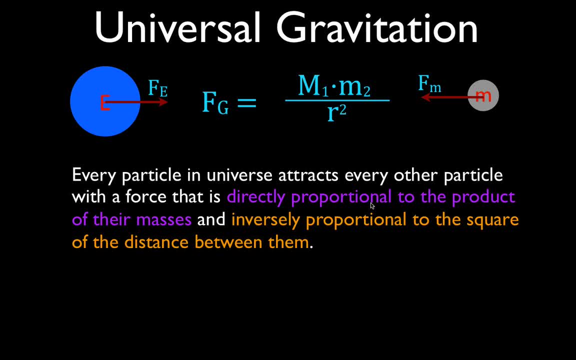 two objects: As the masses increase, the force increases. As the distance increases, the force decreases. Okay, Now they get farther apart. All right now there's one thing missing from this equation, and right here you may notice that there's a space, and we're going to put g in. 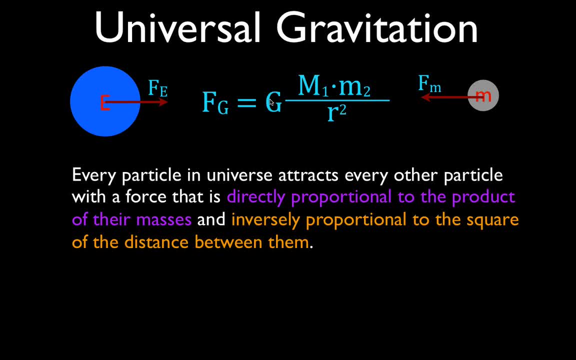 there. That is the gravitational constant, which we'll talk about in the next slide. All right, so there's a couple other things. I just want to point out that the force acts on a straight line between those two objects. So it's just a straight line between those two objects And the magnitude of 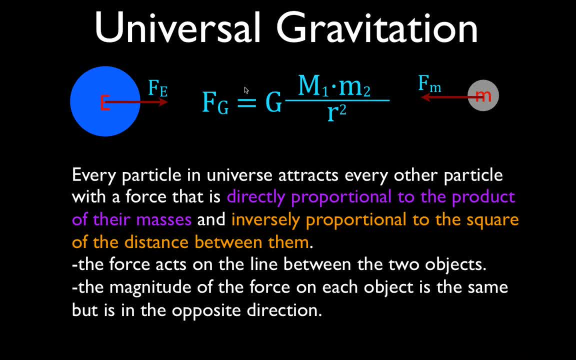 the force on each object is the same, but it acts in the opposite direction. So the magnitude of the force on the earth from the moon is equal to the magnitude of the force on the moon from the earth, But you see, they point in the opposite direction. It's an attractive force. They always attract each other. Okay, 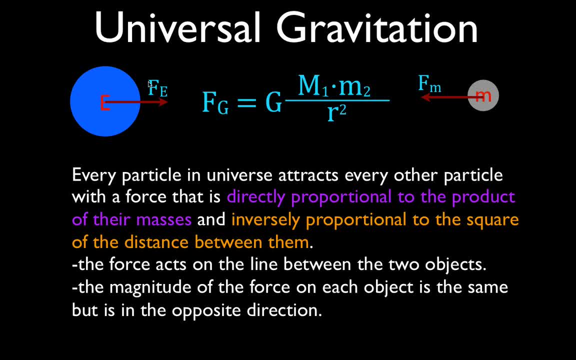 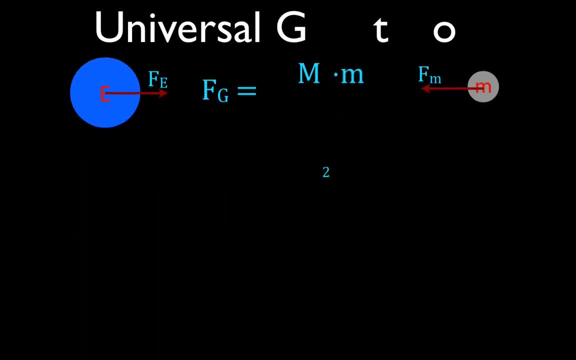 there's no repulsive forces here with the masses and gravitation. So here we have the force on the earth and the force on the moon, and in the next slide we're actually going to use our equation to calculate the amount of force on the earth and the moon. Okay, 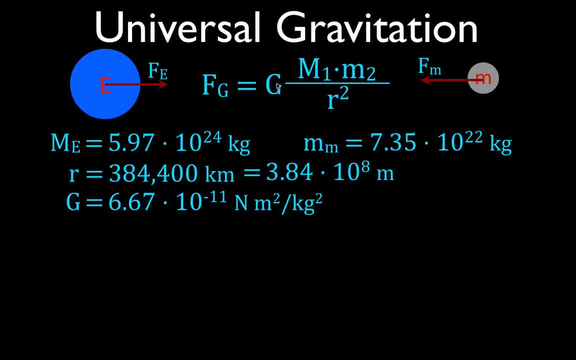 so here's our equation: We have g, which is our gravitational constant, which we'll show you in just a second, as you can see, And we have the mass of the two objects divided by the square of the distance between them. So I'm just going to plug the values in It's. 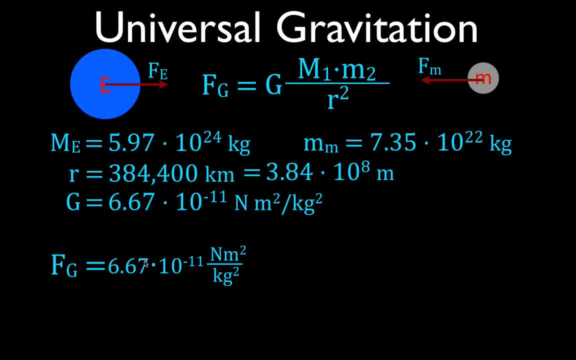 pretty straightforward. We have our gravitational constant. Now you'll notice. the gravitational constant has units of Newton, meter squared, kilogram squared. So this is the mass of the earth, 5.97 times 10. to the 24th kilogram. This is the mass of the moon, 7.35 times 10. 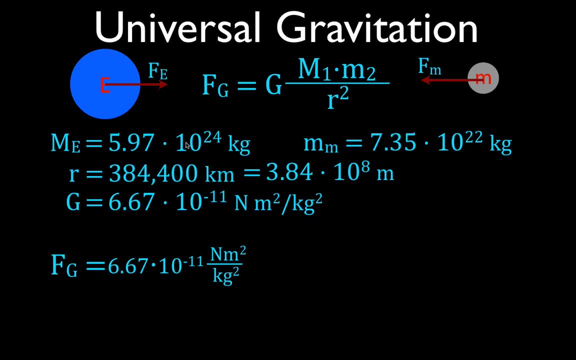 to the 22th kilogram. The masses are typically given in kilograms. If they're not, you have to convert them to kilograms, because that's the units. Now, the distance you can see is often given in kilometers- 384,400 kilometers- But the 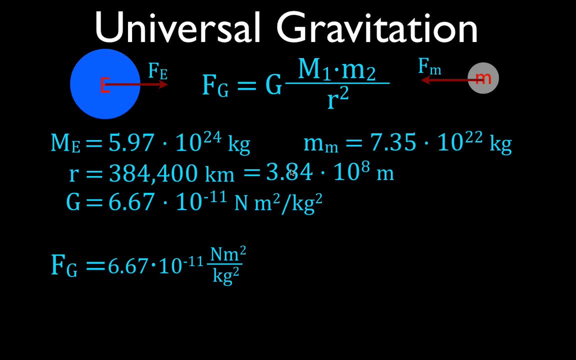 constant has meters. so we have to convert 3.84 times 10 to the 8th meters. The distance must be in meters, The masses must be in kilograms. This is the gravitational constant: 6.67 times 10 to the minus 11.. 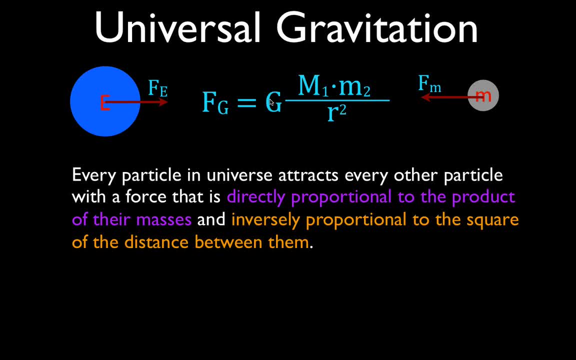 there. That is the gravitational constant, which we'll talk about in the next slide. All right, so there's a couple other things. I just want to point out that the force acts on a straight line between those two objects. So it's just a straight line between those two objects And the magnitude of 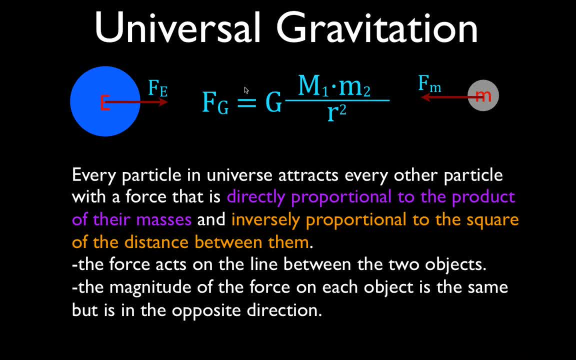 the force on each object is the same, but it acts in the opposite direction. So the magnitude of the force on the earth from the moon is equal to the magnitude of the force on the moon from the earth, But you see, they point in the opposite direction. It's an attractive force. They always attract each other. Okay, 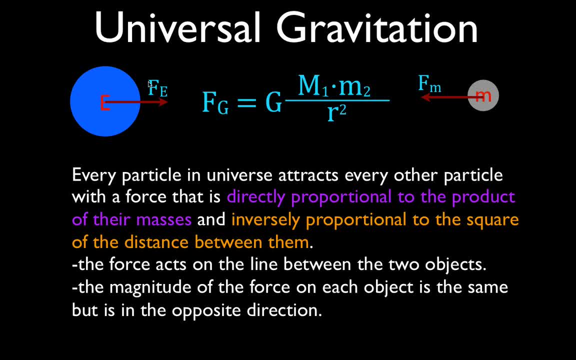 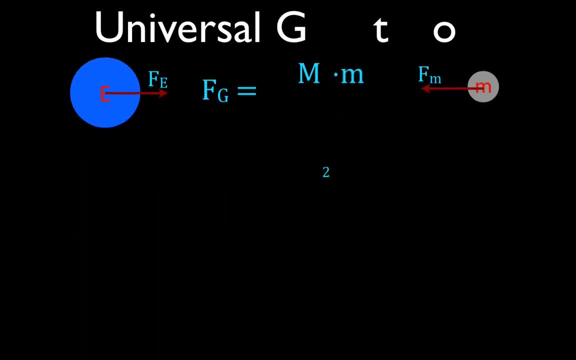 there's no repulsive forces here with the masses and gravitation. So here we have the force on the earth and the force on the moon, and in the next slide we're actually going to use our equation to calculate the amount of force on the earth and the moon. Okay, 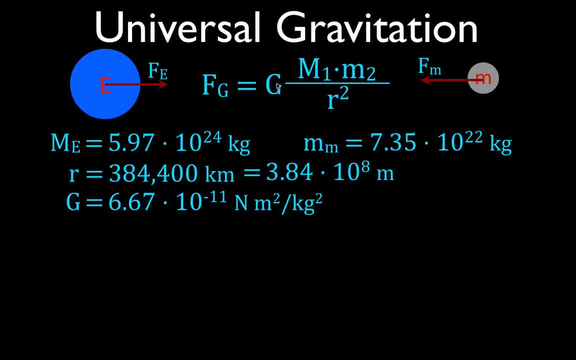 so here's our equation: We have g, which is our gravitational constant, which we'll show you in just a second, as you can see, And we have the mass of the two objects divided by the square of the distance between them. So I'm just going to plug the values in It's. 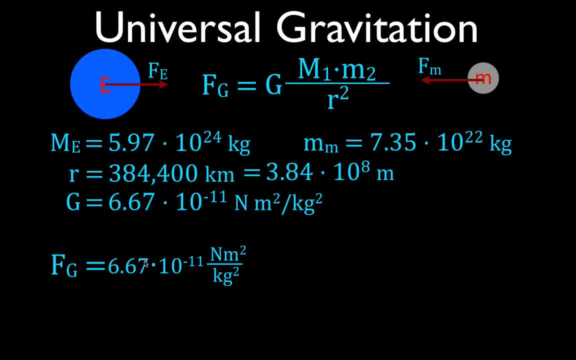 pretty straightforward. We have our gravitational constant. Now you'll notice. the gravitational constant has units of Newton, meter squared, kilogram squared. So this is the mass of the earth, 5.97 times 10. to the 24th kilogram. This is the mass of the moon, 7.35 times 10. 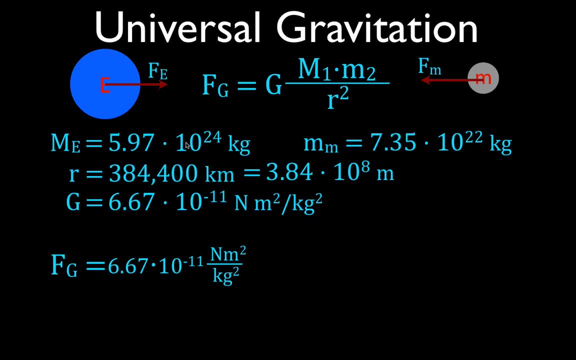 to the 22th kilogram. The masses are typically given in kilograms. If they're not, you have to convert them to kilograms, because that's the units. Now, the distance you can see is often given in kilometers- 384,400 kilometers- But the 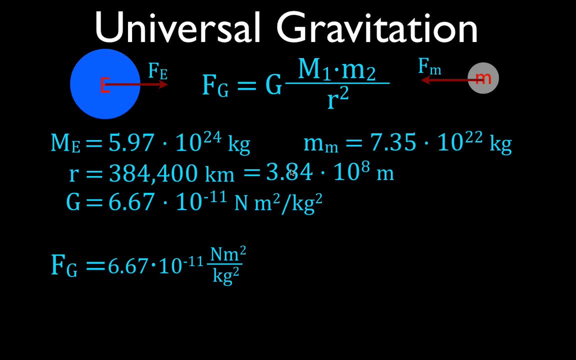 constant has meters. so we have to convert 3.84 times 10 to the 8th meters. The distance must be in meters, The masses must be in kilograms. This is the gravitational constant: 6.67 times 10 to the minus 11.. 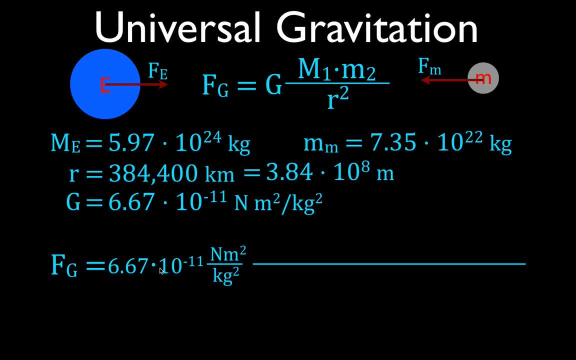 All right, now we're just going to put the values in for the masses, the mass of the earth, the mass of the moon, And we're going to divide that by the square of the distance between them And we come up with that the force of attraction between the earth and the moon is 1.99 times 10 to. 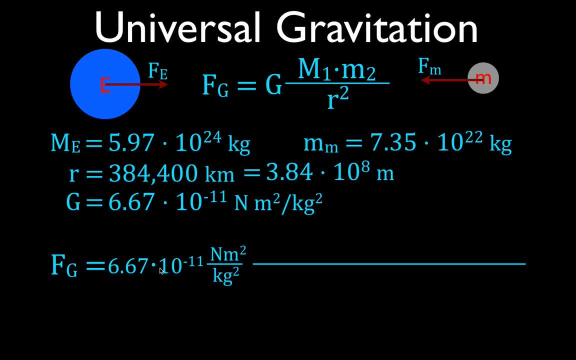 All right, now we're just going to put the values in for the masses, the mass of the earth, the mass of the moon, And we're going to divide that by the square of the distance between them And we come up with that the force of attraction between the earth and the moon is 1.99 times 10 to. 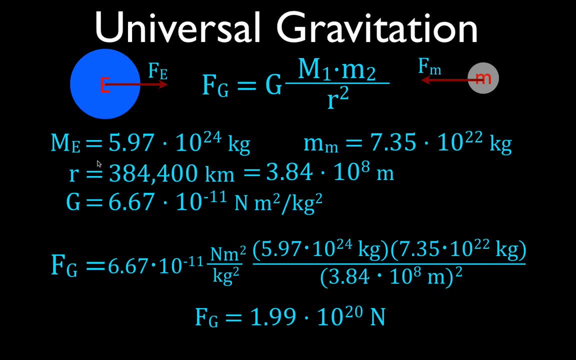 the 20 Newtons. Okay, I just want to point out again that the force, the amount of force on the earth from the moon is 1.99 times 10 to the 20.. The force on the moon from the earth has the same magnitude, so they're both the same. Now sometimes students will ask: 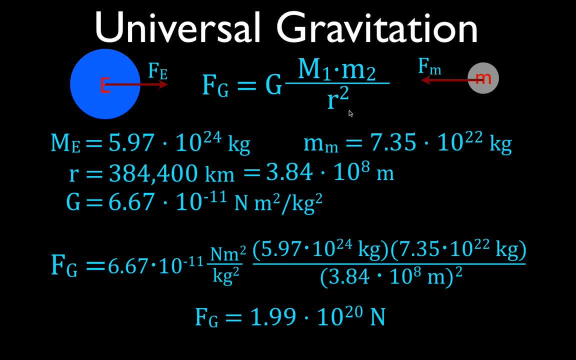 me well, which one is m1 and which one is m2? It doesn't matter. So you just multiply the two values: m1 times m2.. So it doesn't matter which one you put. It doesn't matter if you put the earth's mass here and the moon here, or the earth here and the moon here, because 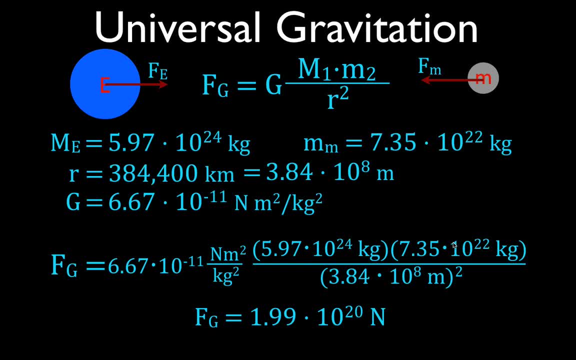 let's just say, for example, this was 3 and this was 2.. 3 times 2 is 6.. Well, if you switch them, this is 3 and this is 2, then 3 times no, 2 and 3.. Well, anyway, it doesn't matter. 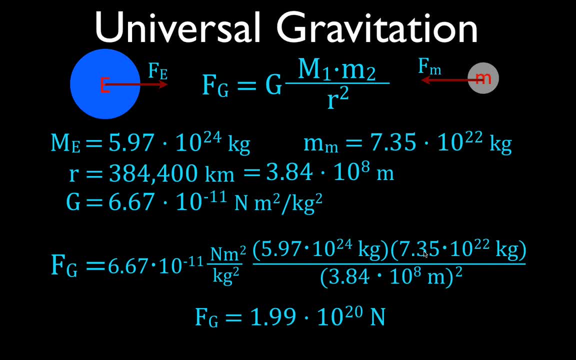 You're just multiplying the two masses, so it doesn't matter which one you put in as m1 and which one you put it in as m2.. You'll notice we have m1.. When we're talking about planets and rotation, typically the 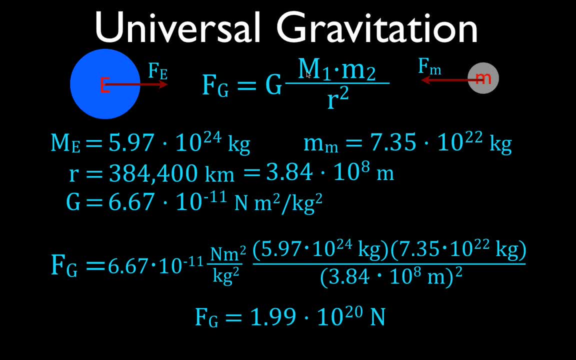 central object I like to use is m1.. So I'm going to put m1 in here, I'm going to put m2 in here, I'm going to put m2 in here. So that's what we're going to need to use is m1 to be consistent. and then the thing 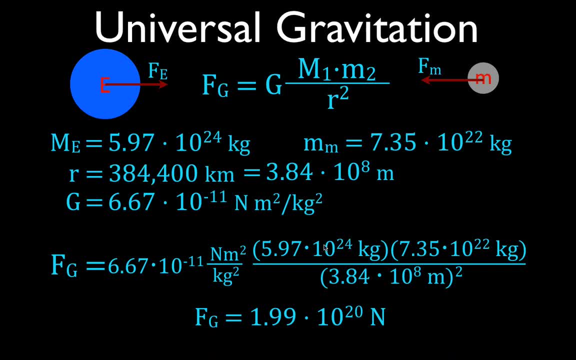 that's orbiting around that central object. we put in as m2, as I did here, earth and moon, Okay, But it doesn't matter. It doesn't matter what order you put them in. You're just multiplying this times, this times, this, divided by the square of the distance between them. 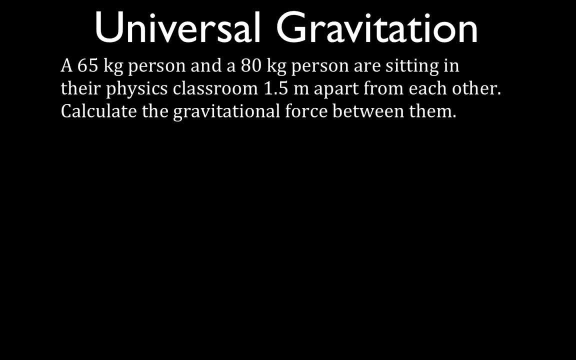 All right, Now let's do a little bit more. interesting problem: maybe Now we have other particles besides the earth and the moon and the planets and the stars. We have people, and people are attracted to each other through their gravitation and through their mass. 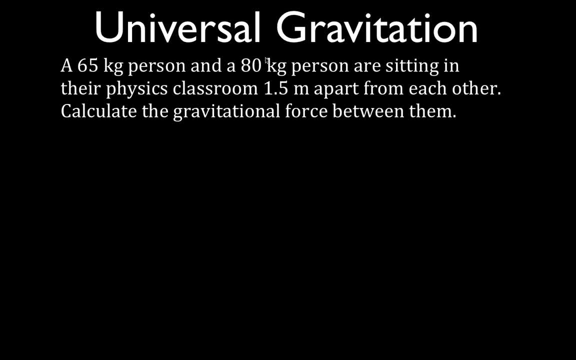 Okay, we have two people. we have a 65 kilogram person and 80 kilogram person. they're sitting next to each other in physics class, but they're separated by a distance of 1.5 meters. they want to calculate the gravitational force between those two objects. those two people get out your equation and we have 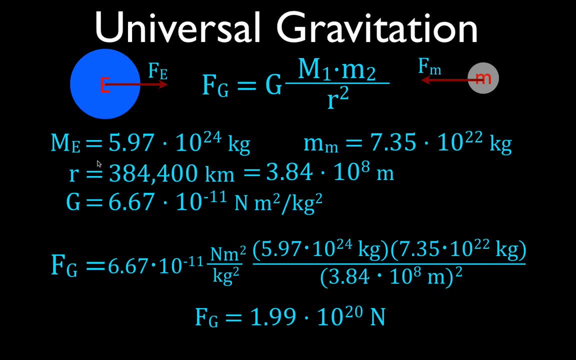 the 20 Newtons. Okay, I just want to point out again that the force, the amount of force on the earth from the moon is 1.99 times 10 to the 20.. The force on the moon from the earth has the same magnitude, so they're both the same. Now sometimes students will ask: 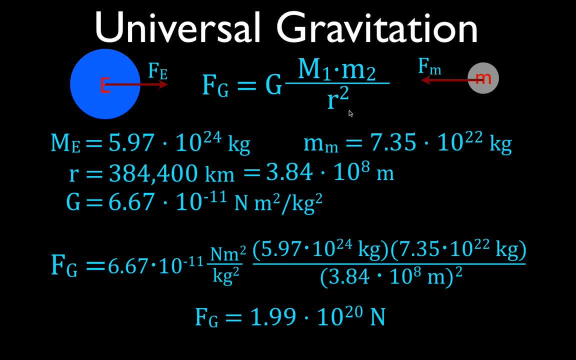 me well, which one is m1 and which one is m2? It doesn't matter. So you just multiply the two values: m1 times m2.. So it doesn't matter which one you put. It doesn't matter if you put the earth's mass here and the moon here, or the earth here and the moon here, because 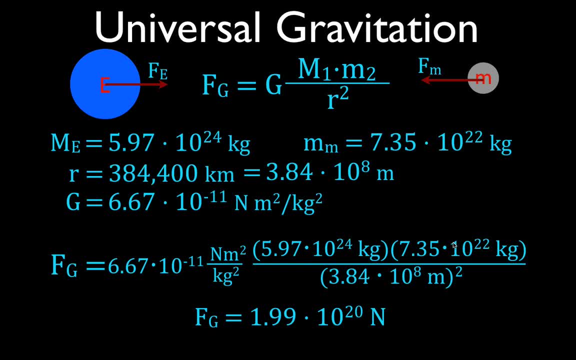 let's just say, for example, this was 3 and this was 2.. 3 times 2 is 6.. Well, if you switch them, this is 3 and this is 2, then 3 times no, 2 and 3.. Well, anyway, it doesn't matter. 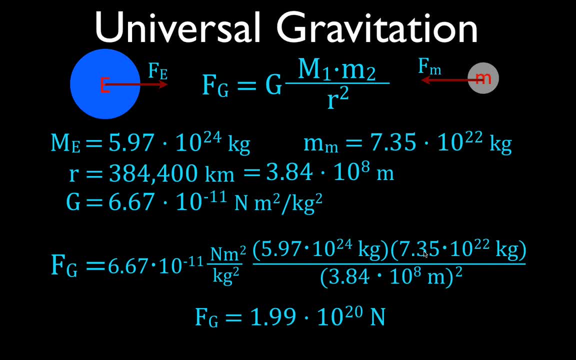 You're just multiplying the two masses, So it doesn't matter which one you put in as m1 and which one you put it in as m2.. You'll notice we have m1.. When we're talking about planets and rotation, typically the central object I like to use is m1.. So I'm going to put m1 in here. I'm going to put m2 in here. I'm going to put m2 in here. I'm going to put m2 in here. I'm going to put m1 in here. I'm going to put m2 in here. 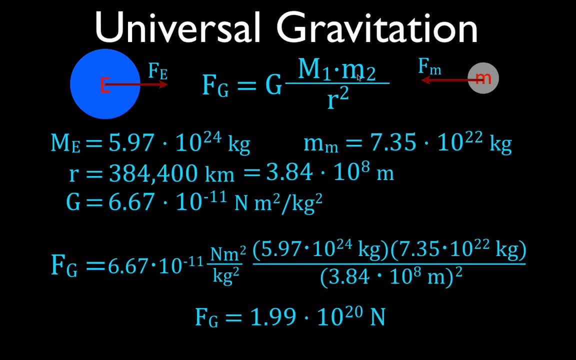 I'm going to put m2 in here. I'm going to put m2 in here, And then we're going to use m1 to be consistent, And then the thing that's orbiting around that central object, we put in as m2, as I did here: earth and moon. 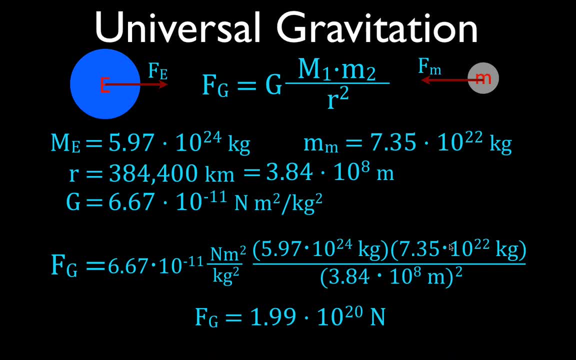 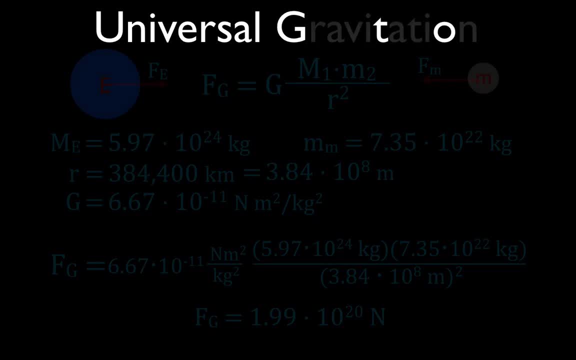 OK, But it doesn't matter. It doesn't matter what order you put them in. You're just multiplying this times, this times this divided by the square of the distance between them. All right, Now let's do a little bit more interesting problem. maybe Now we have other. 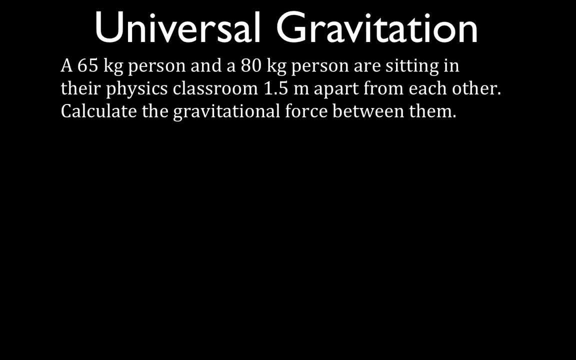 particles. besides the earth and the moon and the planets and the stars, We have people, And people are attracted to each other through their gravitation and through their mass. OK, have two people. we have a 65 kilogram person and 80 kilogram person. they're sitting next to each. 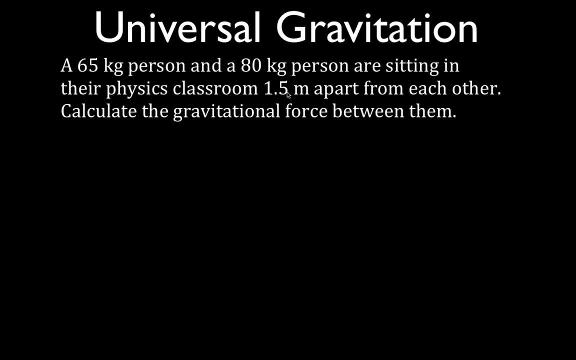 other in physics class, but they're separated by a distance of 1.5 meters. they want to calculate the gravitational force between those two objects. those two people get out your equation and we have the equation: is g, m1, m2, r squared divided by r squared? plug the values in g is same, g doesn't. 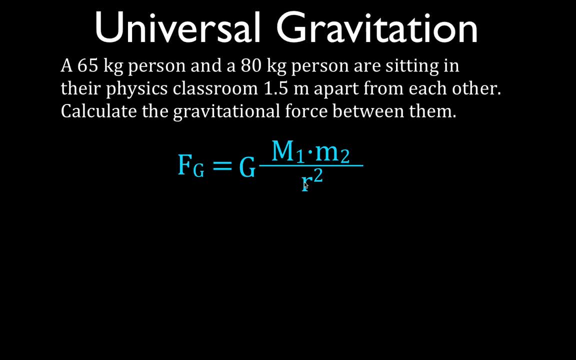 the equation is: g m1 m2 r squared divided by r squared. plug the values. in g is same g doesn't matter what you're talking about, it's still the same. g: 6.67 times 10 to minus 11 times the mass of.